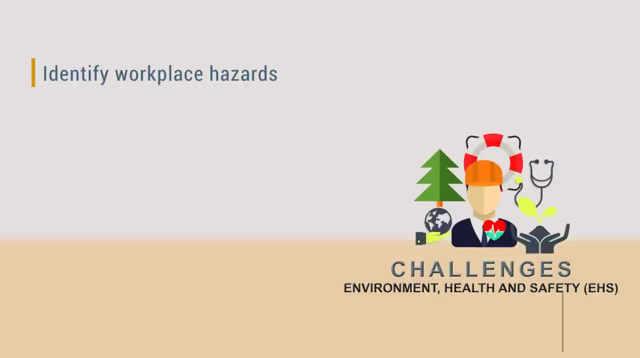 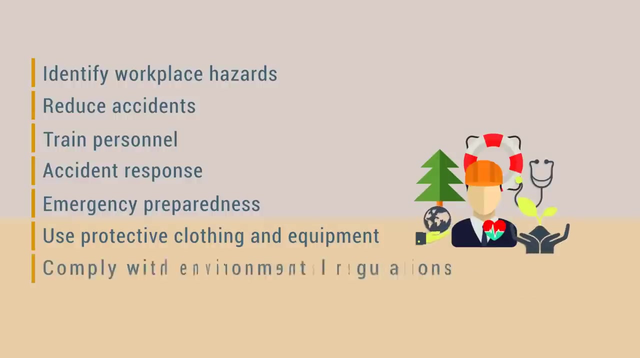 measures and procedures for identifying workplace hazards and reducing accidents and exposure to harmful situations and substances. training of personnel in accident prevention, accident response, emergency preparedness and use of protective clothing and equipment. creating a systematic approach to complying with environmental regulations, such as managing waste or air. 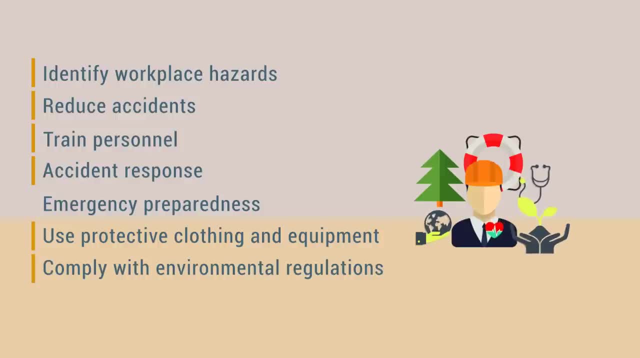 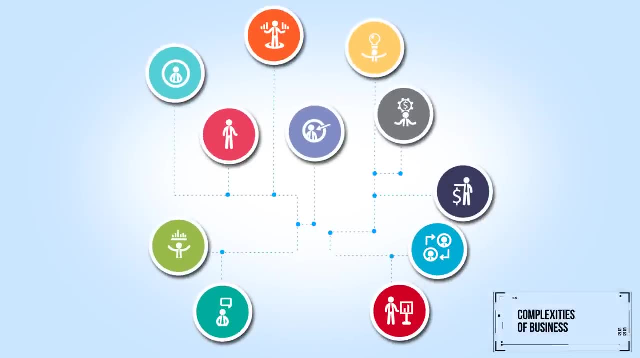 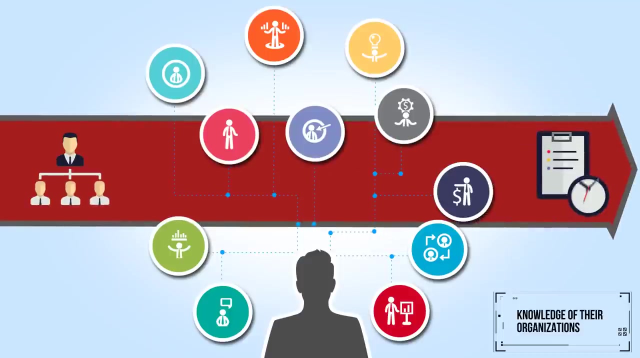 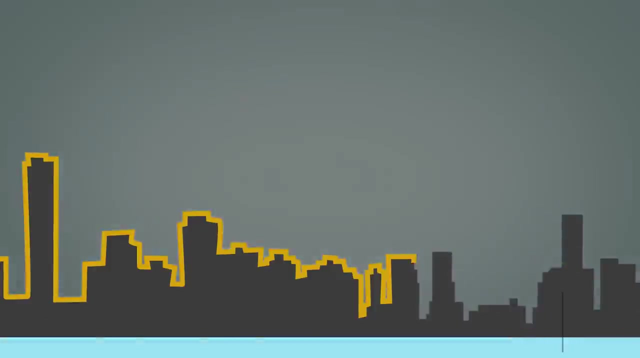 emissions and reducing the company's carbon footprint. As the complexities of business grow, so the depth and scope of EHS teams' knowledge of their organizations, from management level to day-to-day operations, becomes an increasingly valuable resource, providing the opportunity for the function to expand beyond legal and 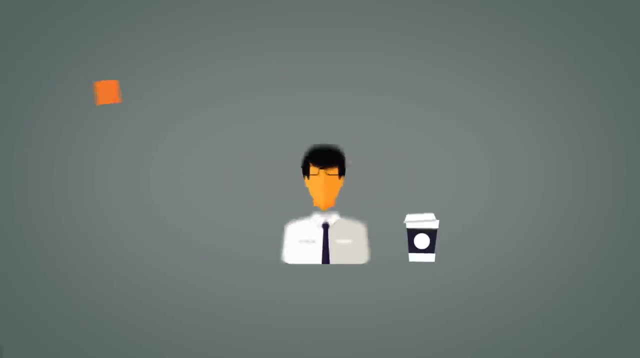 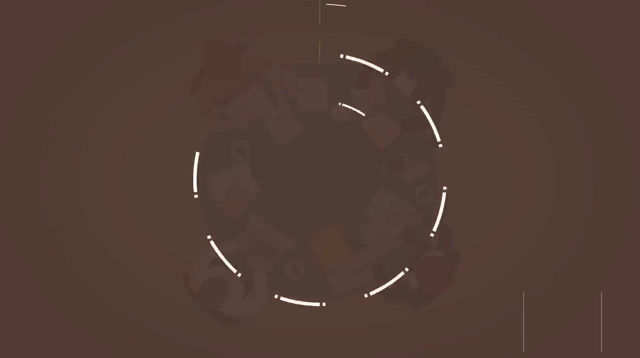 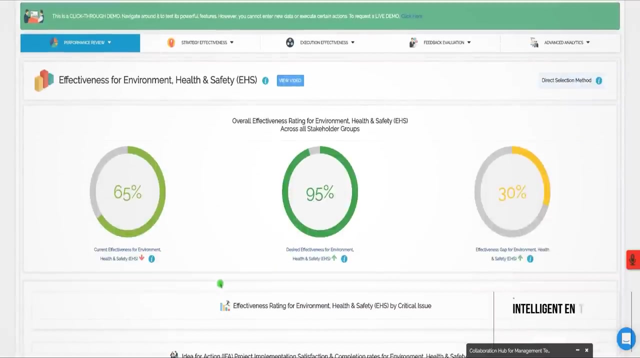 regulatory compliance and risk control to facilitating sustainability, corporate citizenship and customer-centric business. But EHS often fails to deliver its intended benefits because of a lack of 360-degree stakeholder intelligence, cognitive insights and real-time performance management capabilities. Performax 360 is an intelligent enterprise performance management platform that helps. 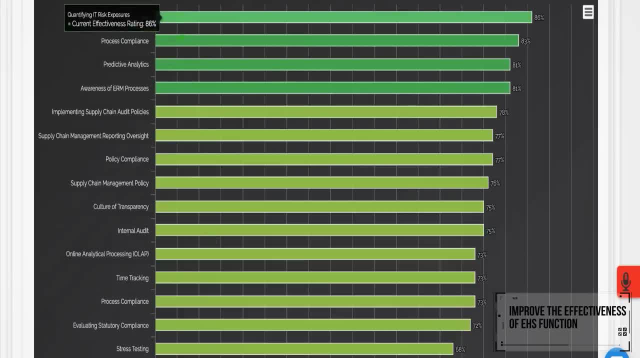 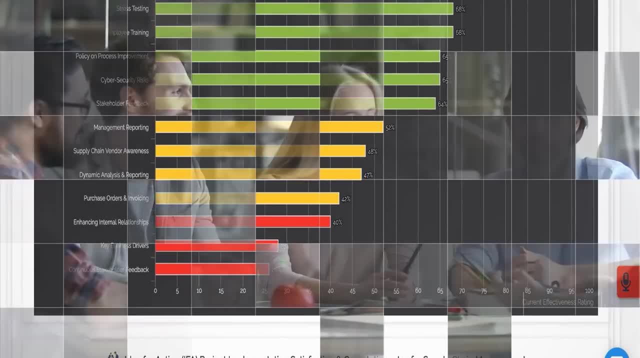 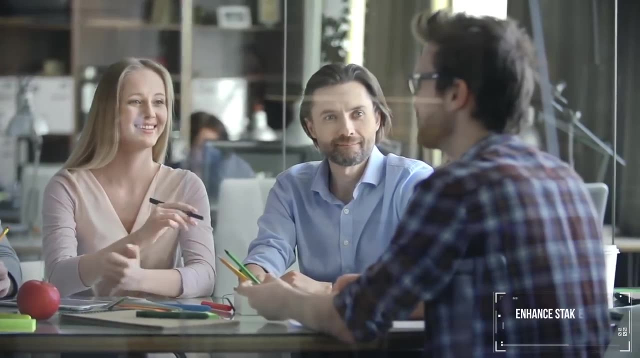 improve the effectiveness of the EHS function by providing the best possible performance management capabilities for all, By ensuring continuous touchpoints and alignment with key stakeholders. By giving key stakeholders a voice on issues that are critical to the EHS function, you'll enhance stakeholder engagement and spur innovation. 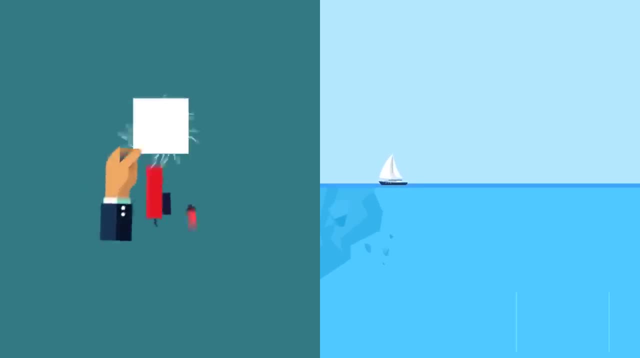 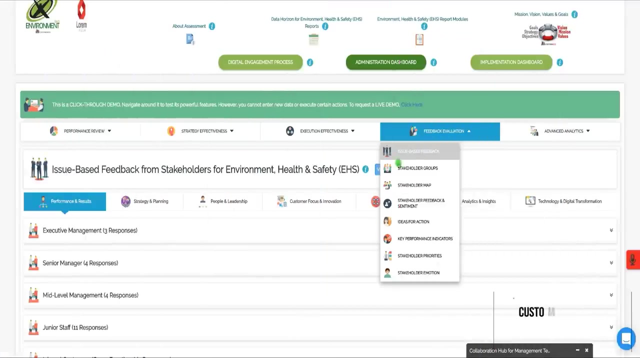 Uncover hidden risks within EHS through unfiltered operational intelligence and actionable insights. Fully customizable and scalable EHS is the best way to improve the performance of your organization By making the organization more scalable. Performax 360 serves as a GPS navigation system for. 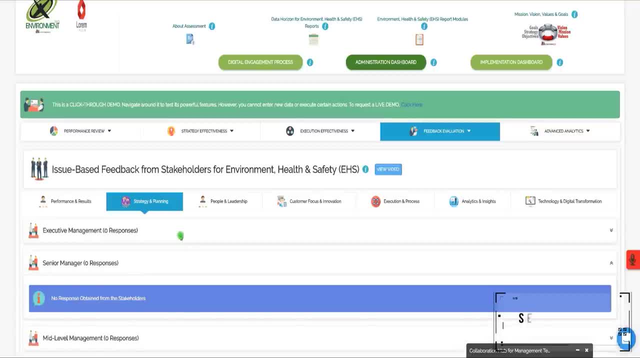 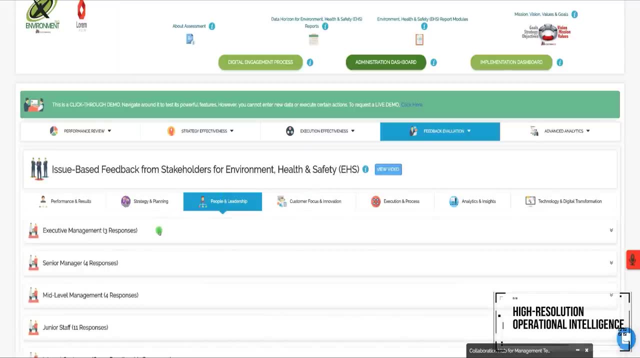 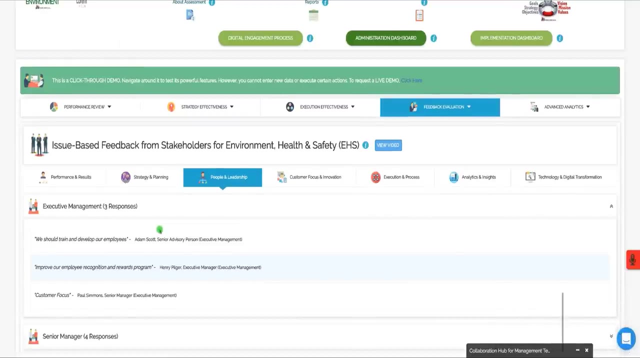 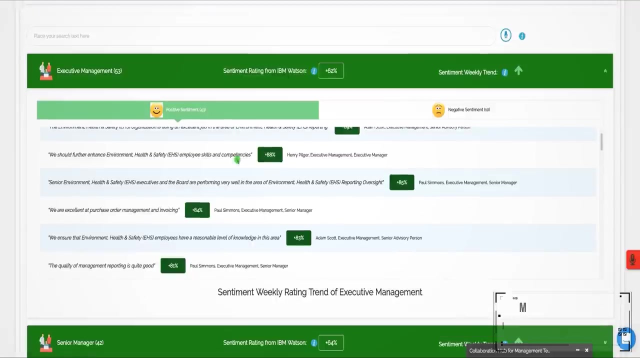 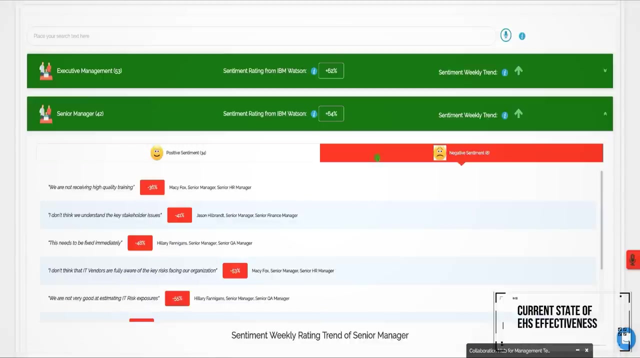 the EHS function that helps you sense and respond with high-resolution operational intelligence from all areas of the enterprise on all critical issues, Supported by IBM Watson Cognitive Analytics By engaging key stakeholders in an ongoing and live feedback process, gain a more accurate and objective 360-degree perspective on the current state of EHS effectiveness. 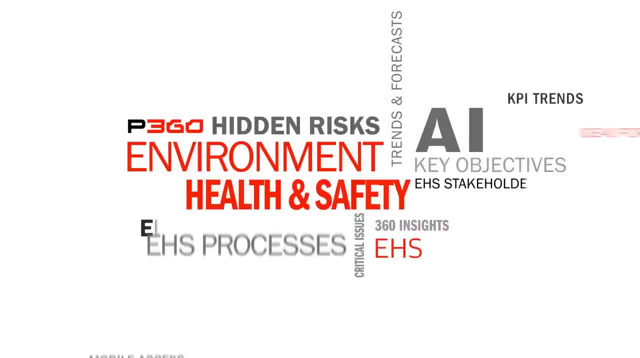 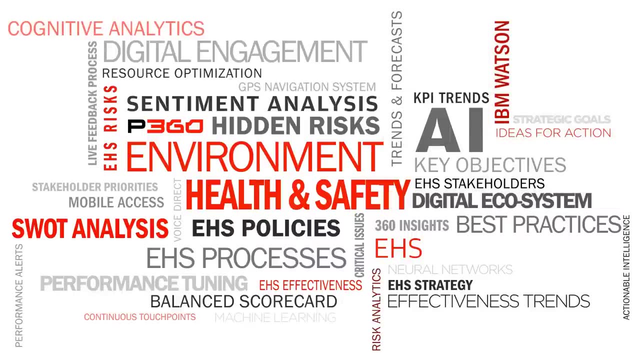 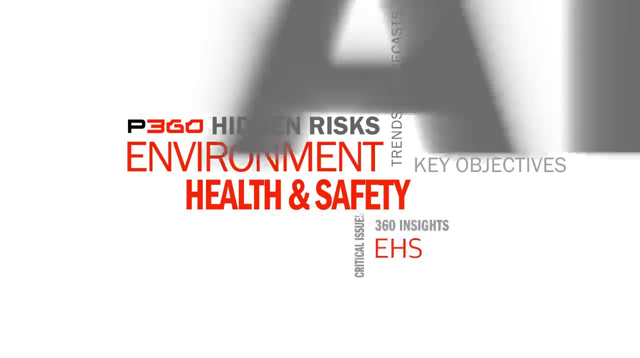 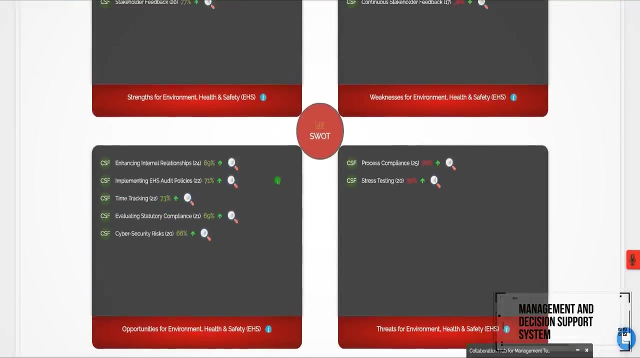 By capturing real-time stakeholder feedback on issues that are critical to the EHS function, Performax 360 helps you see in higher fidelity so you can continually enhance functional effectiveness, agility and responsiveness As a management and decision support system powered by Cognitiv Performax 360 diagnoses. 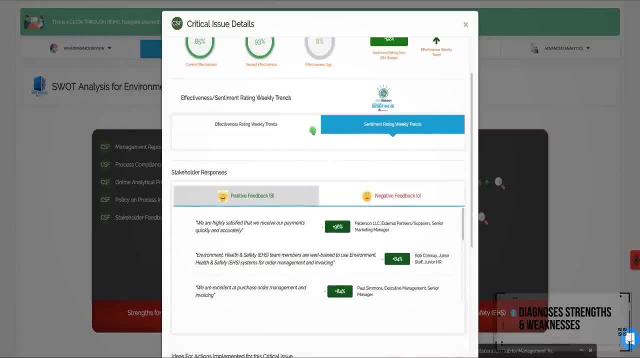 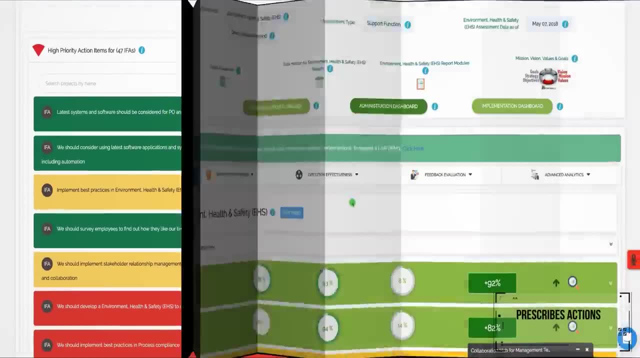 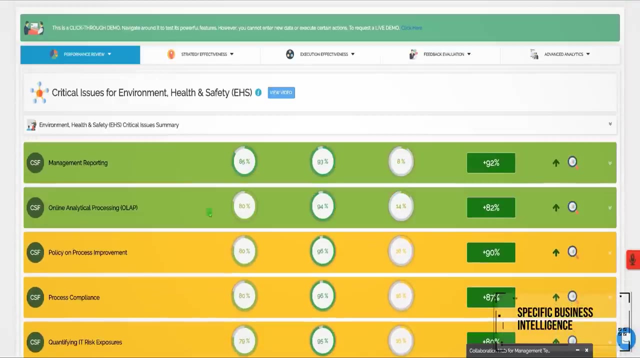 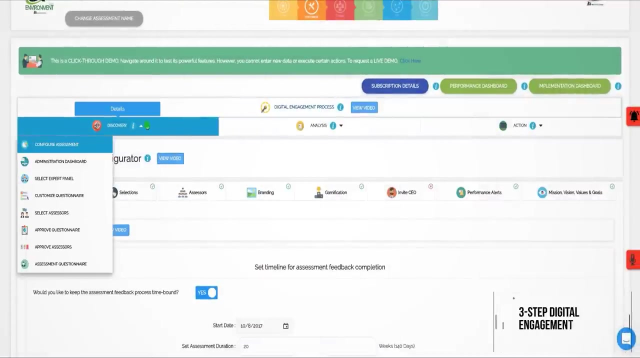 strengths and weaknesses within the existing EHS environment and prescribes actions aligned to stakeholder expectations. Thus, it captures the specific business intelligence you need from key EHS stakeholders and helps you make more informed decisions. There's a three-step digital engagement process for EHS that comprises knowledge discovery. 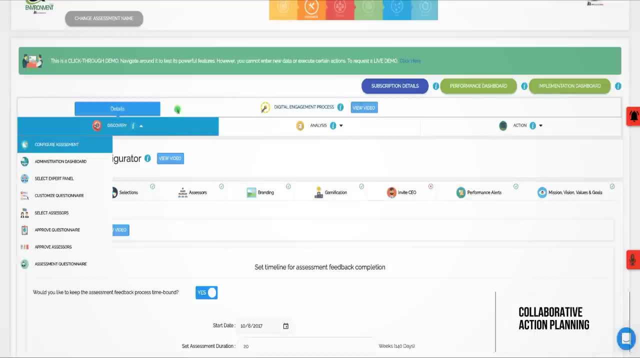 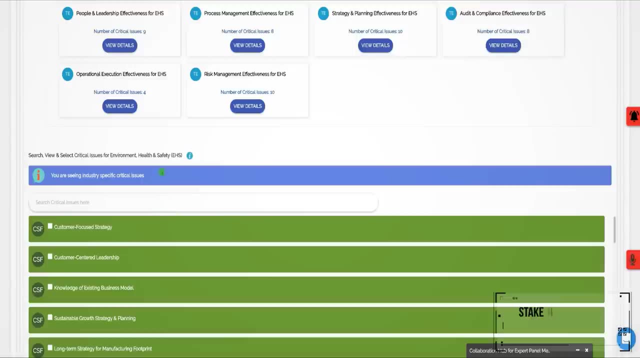 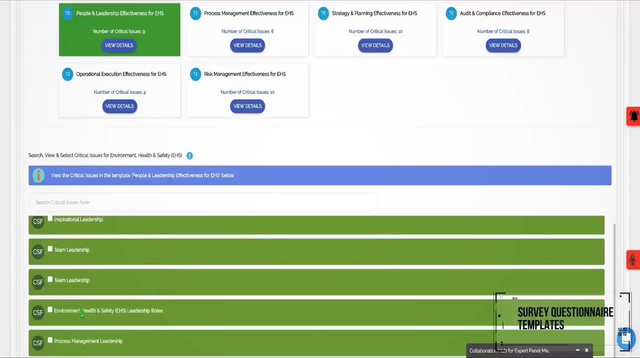 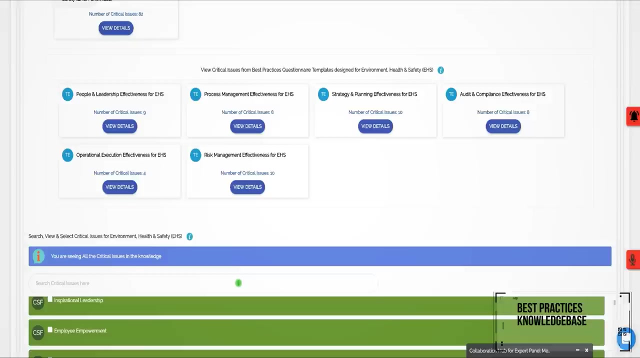 data analytics and collaborative action planning. An expert panel identifies the critical EHS issues on which stakeholder feedback is collected. This is supported by our customizable EHS system. Performax 360 includes a built-in best practices knowledge base with more than 1,000 critical 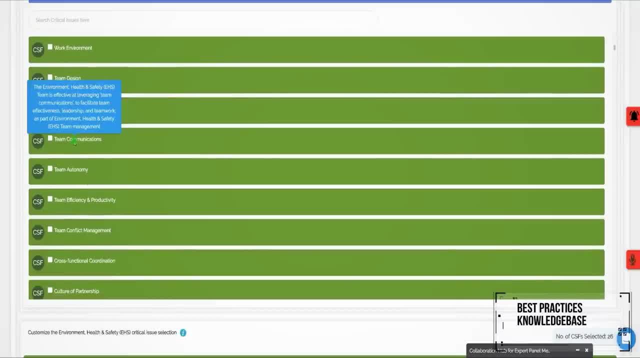 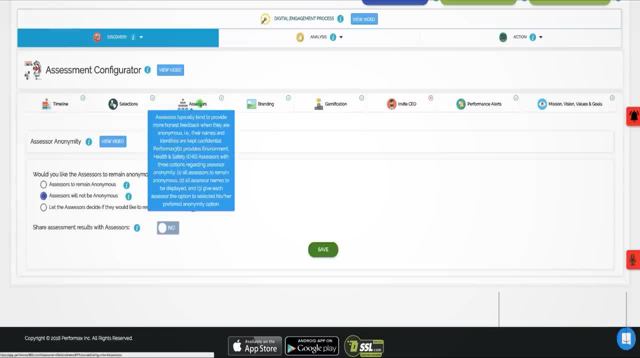 EHS issues and more than 25,000 best practices ideas for action. When EHS team members and internal stakeholders provide feedback, they may choose to remain anonymous throughout the live and ongoing feedback process. Performax 360 is a well-deserved tool for the EHS community. 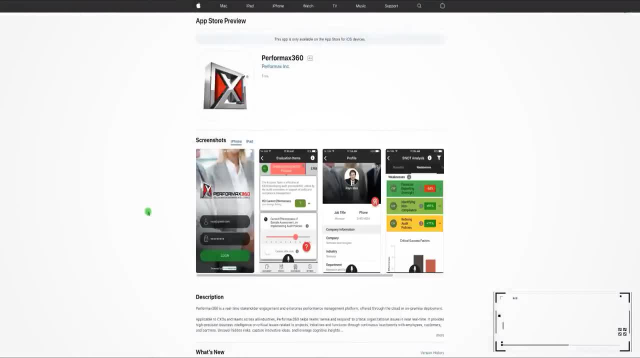 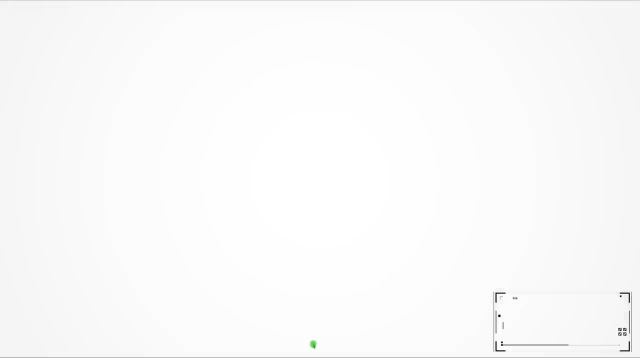 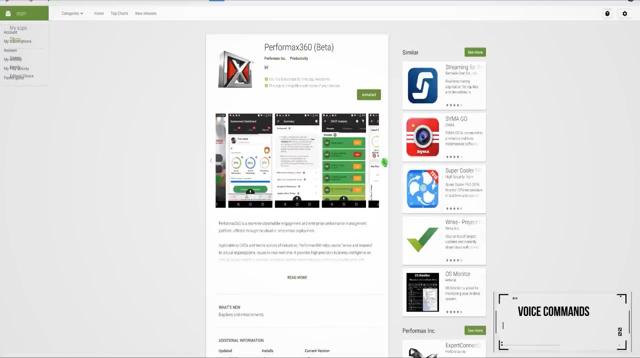 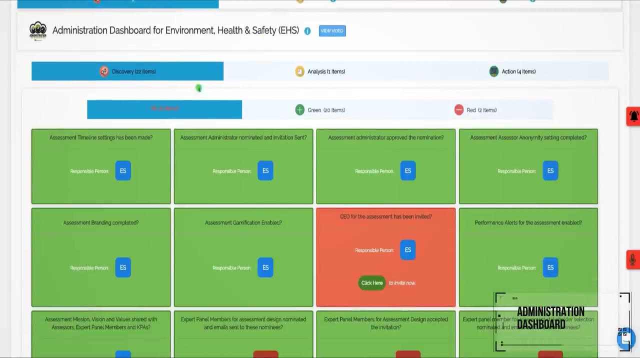 Feedback may be provided using our web platform or mobile iOS and Android apps. The Voice Direct feature allows EHS stakeholders to submit their feedback through voice commands anytime and from anywhere. The Administration Dashboard is designed to help the assessment administrator monitor the assessment implementation progress throughout the three-step digital engagement process. 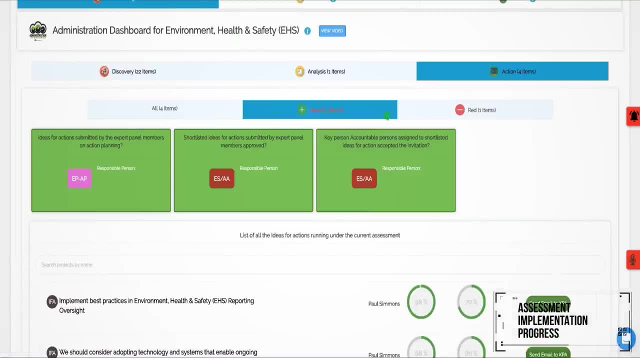 Performax 360 is a well-deserved tool for the EHS community. Performax 360 is a well-deserved tool for the EHS community. The Administration Dashboard is designed to help the assessment administrator monitor the assessment implementation progress throughout the three-step digital engagement process. 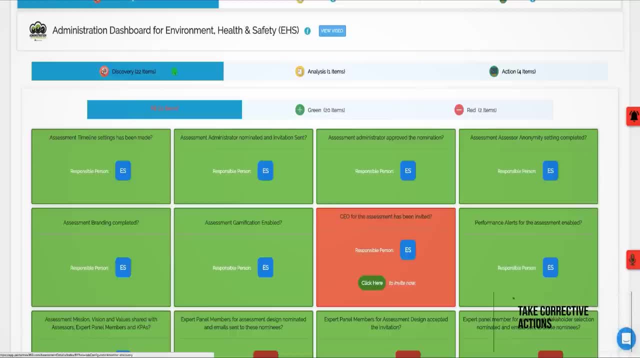 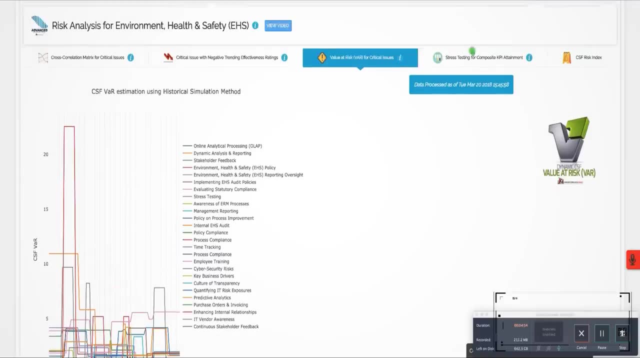 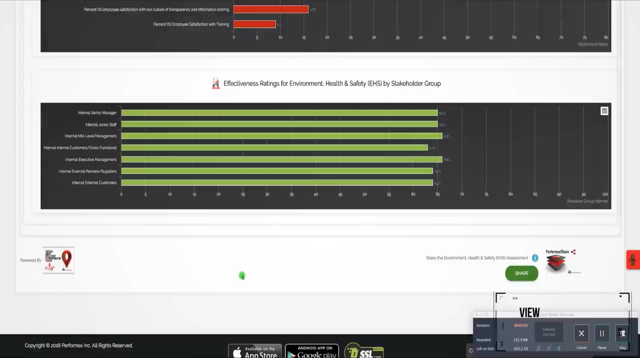 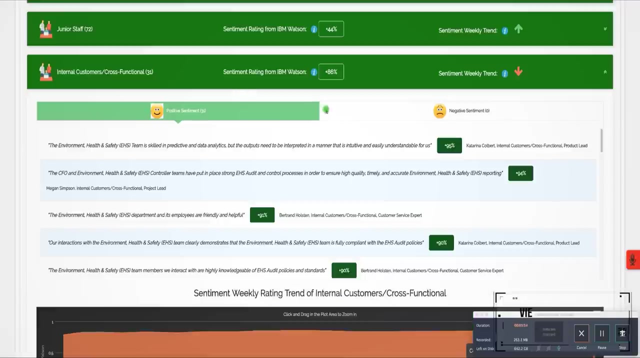 and take corrective actions as required. With more than 30 visual analytics features, the Performance Dashboard leverages state-of-the-art data, science and artificial intelligence. View EHS Effectiveness Ratings and Trends by Stakeholder Group and by Critical Issue. View EHS Stakeholder Sentiment and Emotion Analysis by Stakeholder Group and by Critical 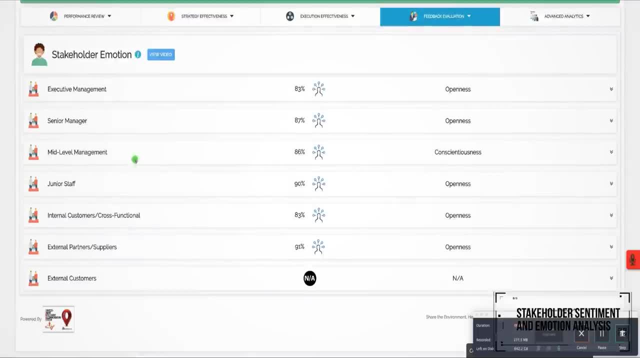 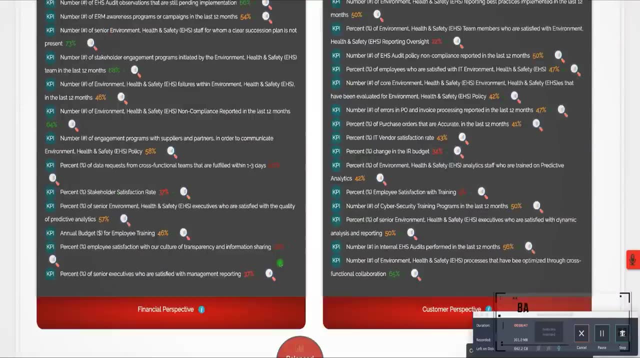 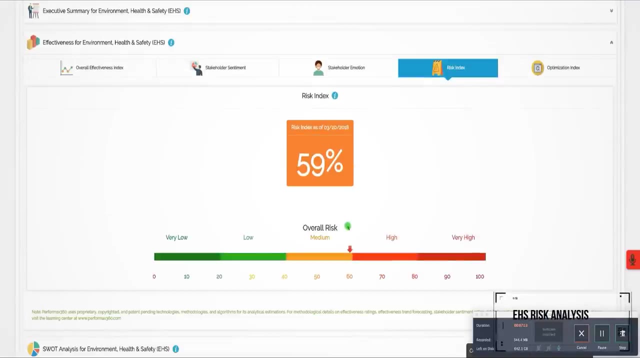 Issue View: EHS Stakeholder Sentiment and Emotion Analysis by Stakeholder Group and by Critical analysis powered by IBM Watson. Examine the dynamic EHS SWOT analysis and balanced scorecard with drill-down details. The EHS risk analysis features an overall functional risk index. highlights negative. 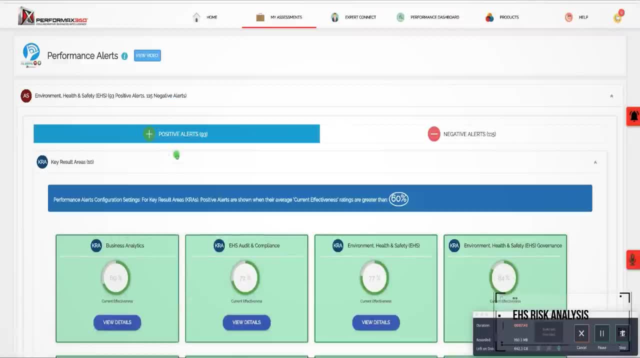 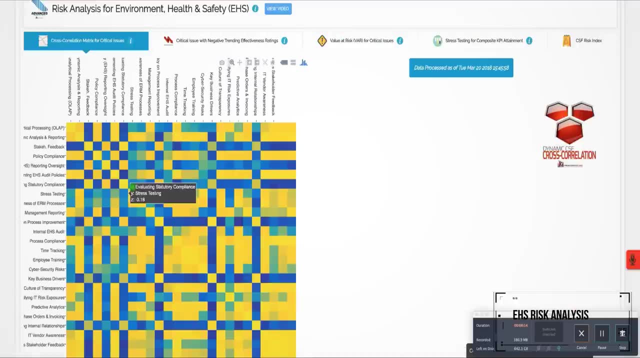 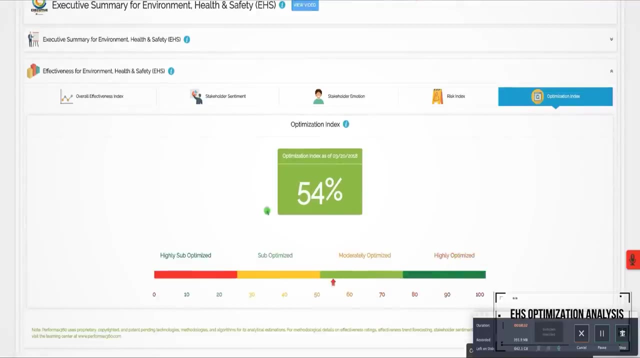 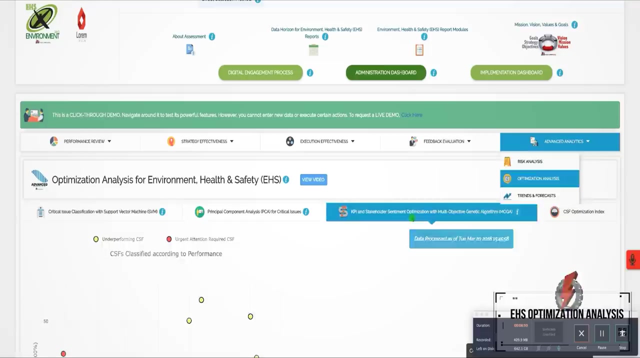 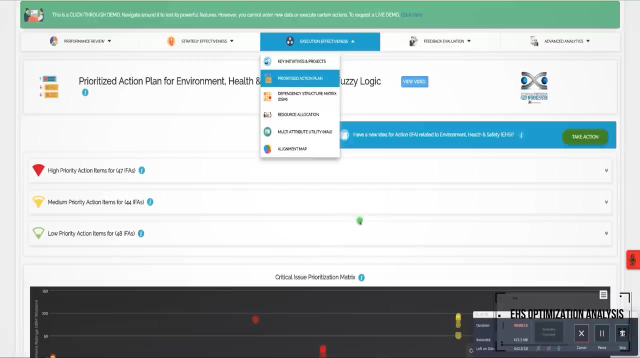 trending areas, provides positive and negative performance alerts and performs value-at-risk analysis, stress testing and correlation analysis. The EHS optimization analysis calculates the functional performance optimization index, evaluates resource allocation optimization, presents KPI optimization and prioritizes key EHS action plans based on artificial intelligence and inputs from subject matter experts. 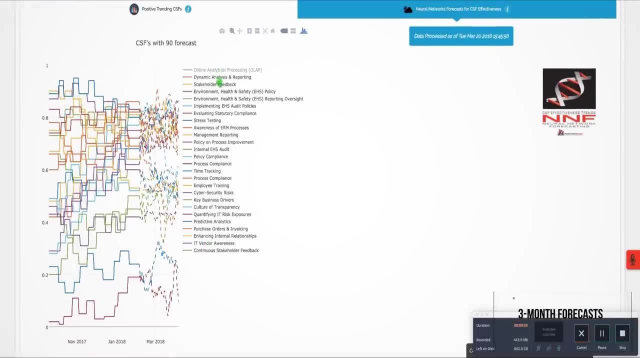 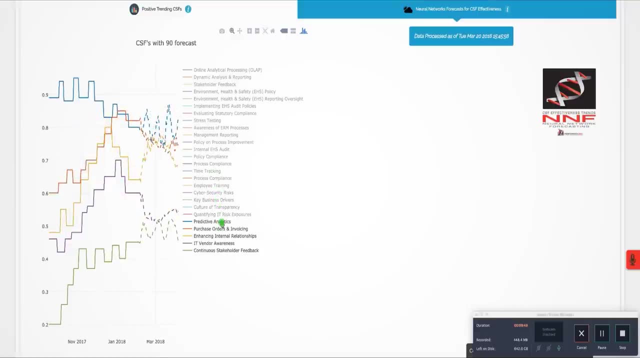 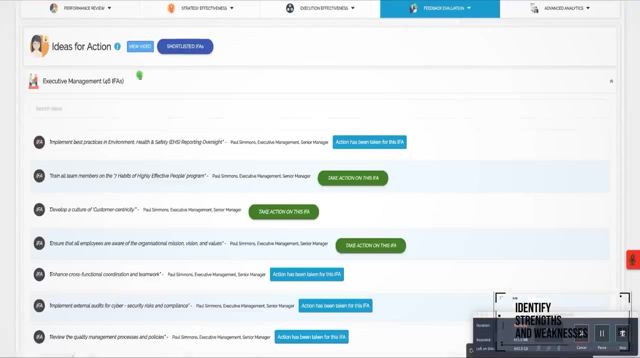 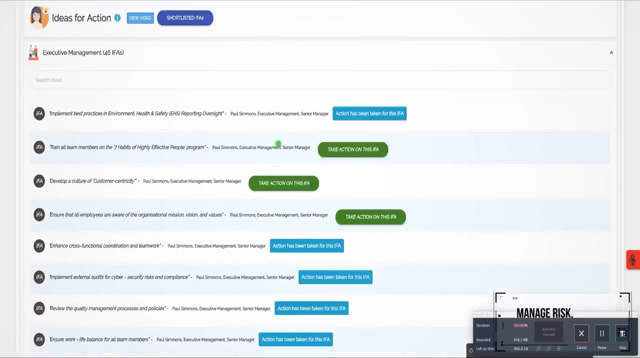 EHS SWOT analysis. In addition, three-month forecasts are provided on the effectiveness ratings of key factors relevant to EHS leveraging neural network forecasting. Key stakeholders not only help identify EHS strengths and weaknesses, they collaboratively recommend ideas for action that help manage risk, spur innovation within the EHS environment. 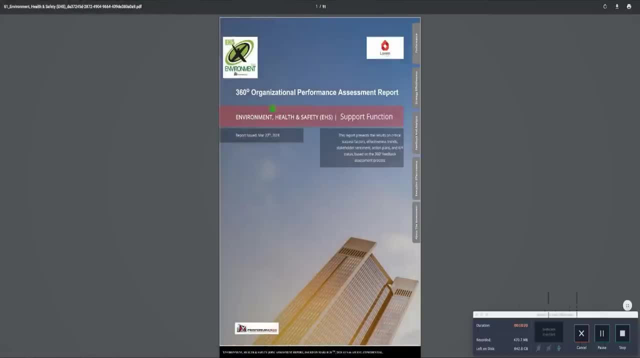 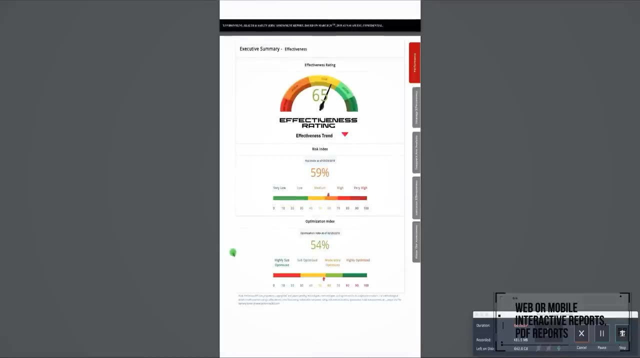 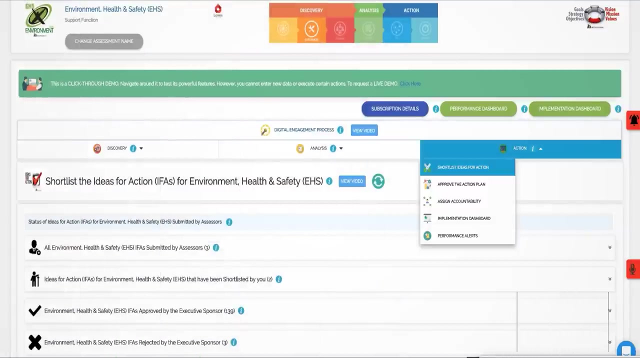 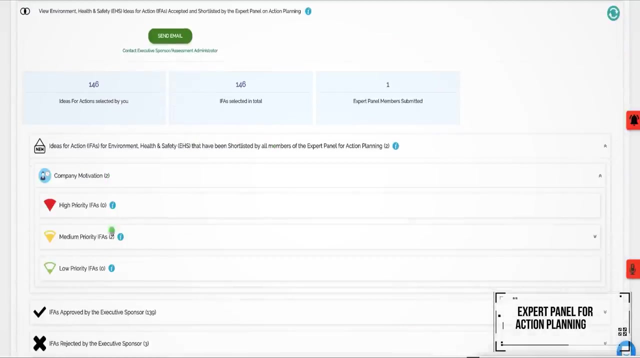 and take actions Where needed. Access EHS performance results 24-7 through web or mobile interactive reports, pdf reports or PowerPoint presentations. An expert panel for action planning reviews stakeholder recommendations, prioritizes them and submits them for approval by the executive sponsor or head of Environment, Health and.